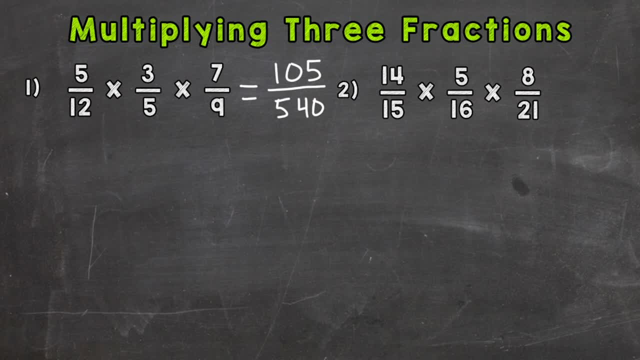 opinion, cancellation makes these problems a lot more manageable and smaller numbers in value that are easier to work with. So let's use cancellation here and we'll notice the difference between the two methods: 12 times 3, fifths times 7, ninths. So when we use cancellation, we look for common factors between the 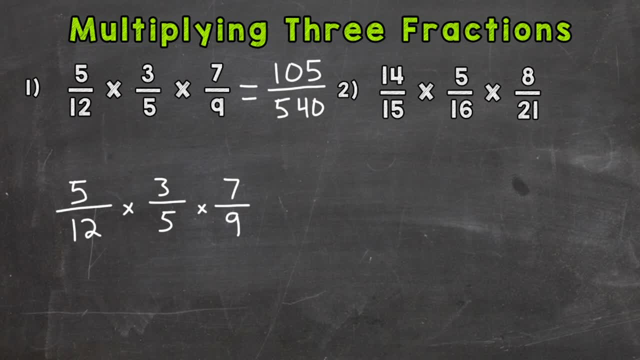 numerators and denominators. You can think of it as simplifying the problem before we multiply and we can use any of the numerators with any of the denominators. So, for example, we can see that we have a 5 here and a 5 here, So a common factor. 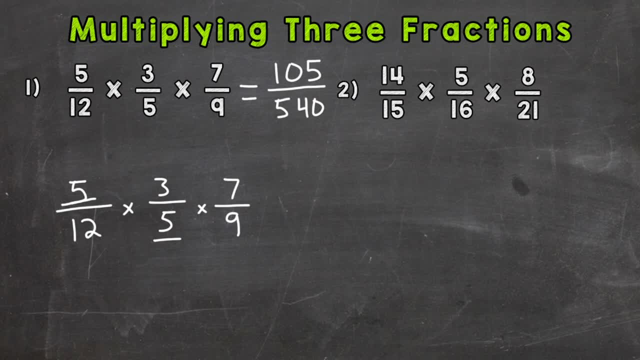 between 5 and 5 is 5.. So let's divide each of those by 5.. 5 divided by 5 is 1, and 5 divided by 5 is 1.. Now we could go from there and multiply straight across, and that's going to be more manageable and simpler than what we did originally- multiplying straight across- and that 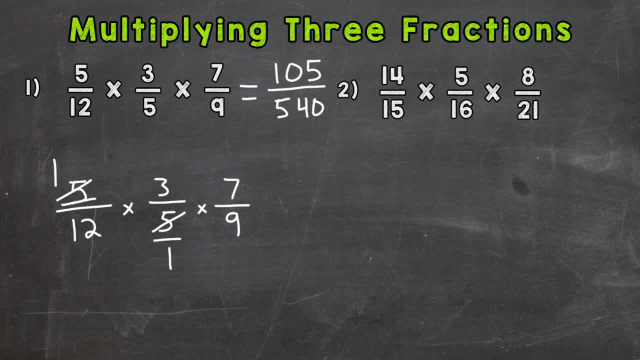 would be fine. But let's see if we have any other common factors. So, for example, we could see that we have a 3 here which will match with this 12 or this 9- here I'm going to use it with the 9.. So a common factor between 3 and 9 is 3. let's divide them both by 3.. So 3 divided by 3 is 1 and 9 divided by 3. 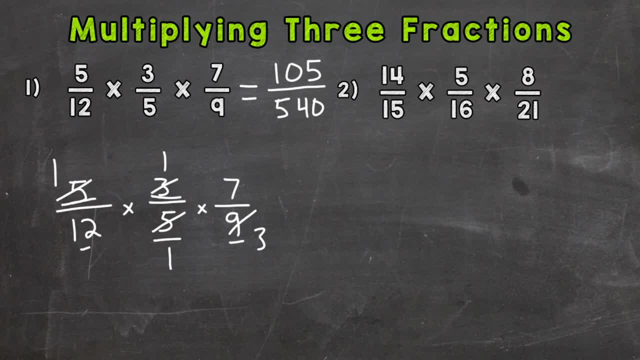 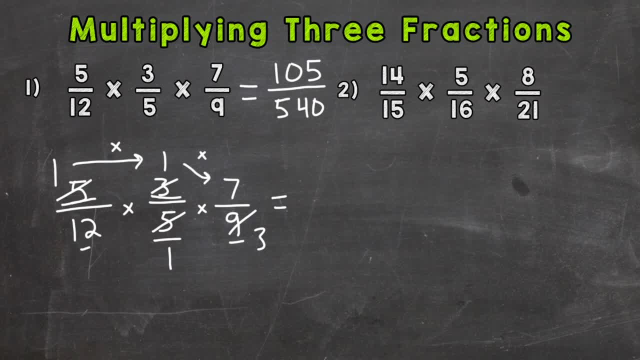 1 times 7.. So 1 times 1 is 1 times 7 is 7.. 12 times 1 is 12 times 3 is 36.. So we get 7 over 36, which is in simplest form. The only common factor between 7 and 36 is 1.. So we are done here. Now I 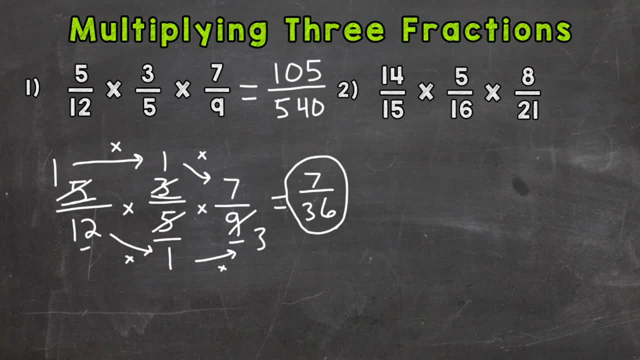 went straight across there without rewriting the problem, which is fine, or you can rewrite the problem to be a little neater and to make everything a little more clear. So let me rewrite here so I can show you what I'm talking about. We have a 1 over 12 times 1 over 1 times. we have a 7. 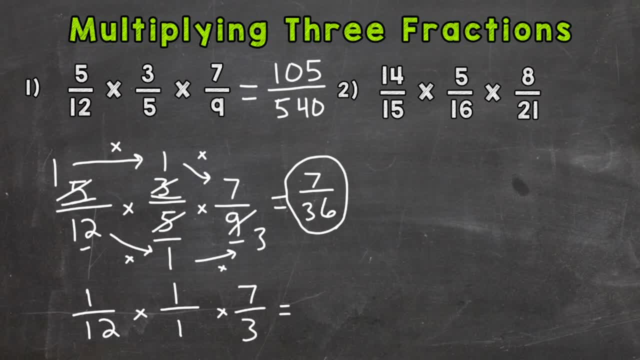 over 3.. So 1 times 1 is 1 times 7 is 7.. 12 times 1 is 12 times 3 is 36.. So I just rewrote the problem there so we can see a little bit better. 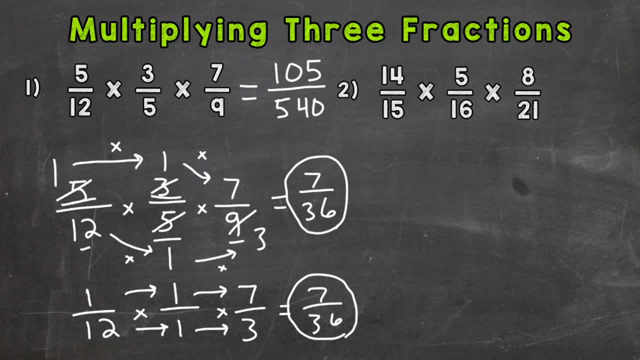 After cancellation, which numbers we were working with. So you can see that we had much smaller, easier and manageable numbers to work with, instead of that original problem where we had 5 times 3 times 7 and 12 times 5 times 9.. Now, if we were to simplify this up here- 105 over 540- we would. 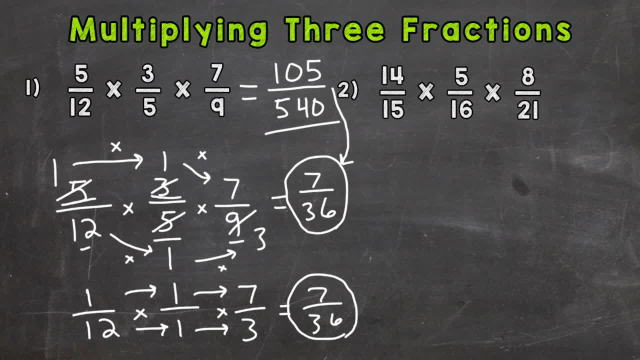 eventually get to 7 over 36.. But it's just much easier to use cancellation and simplify before multiplying in order to get that answer right away. So on to number 2, where we have even larger numbers that we're working with. So if we were to go straight across- which you can do- you can do 14. 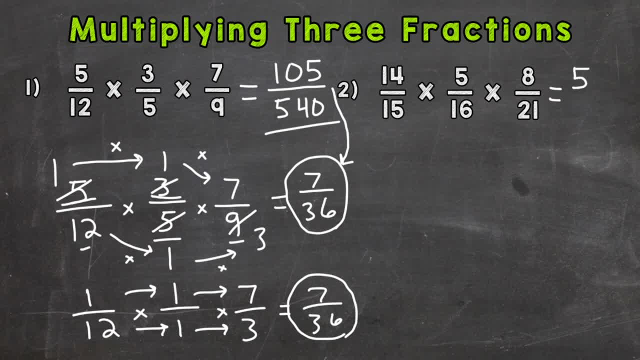 times 5 times 8 and you would end up with 560.. I solved that ahead of time for time's sake here. And the bottom, the denominators: 15 times 16 times 21, we would get 40. Now those are pretty large numbers in value there that we would have to simplify. 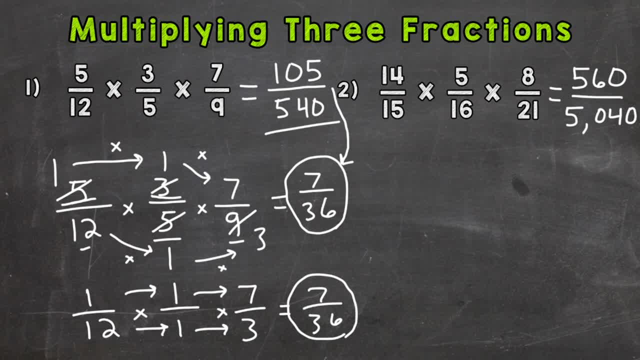 Let's use cancellation in order to make this a little more simple and manageable. So I'm going to rewrite the problem: 14 15ths times 5, 16ths times 8 over 21.. All right, so again we need to look at our numerators and denominators to see if we have any common factors between them. So